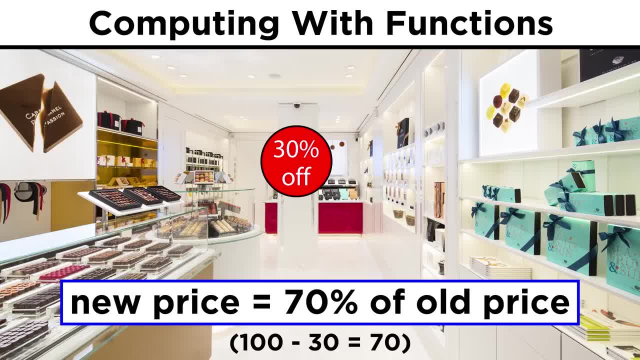 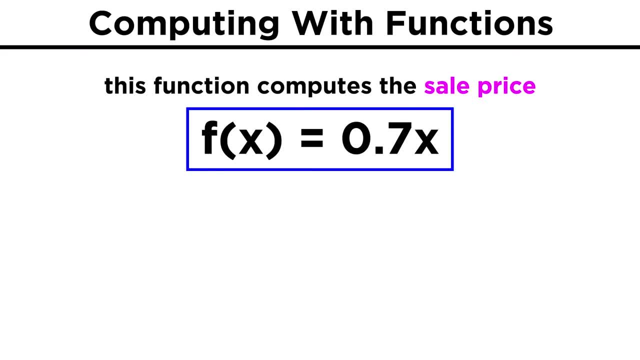 same thing as thirty percent off, since one hundred minus thirty is seventy. The function that we would therefore use to compute the sale price of any item would be: f equals zero point seven x. F is the function, and the x in parentheses, which is read of x, means that the function 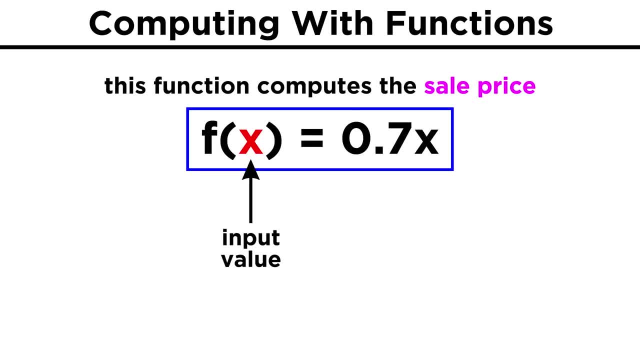 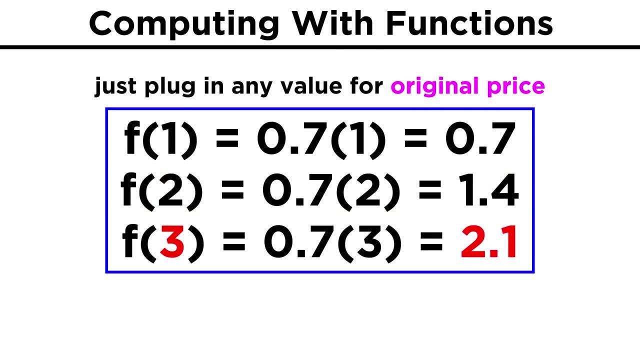 will operate on any x value that you plug in. If we plug in one dollar for x, the function spits out seventy cents. so f of one equals zero point seven. F of two equals one point four. F of three equals two point one. 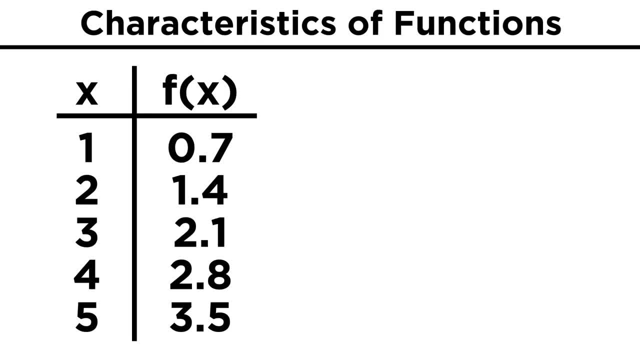 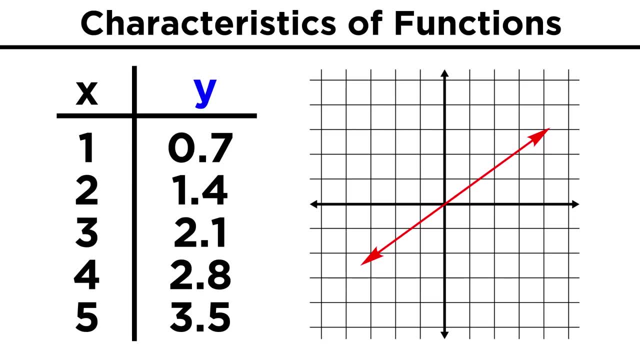 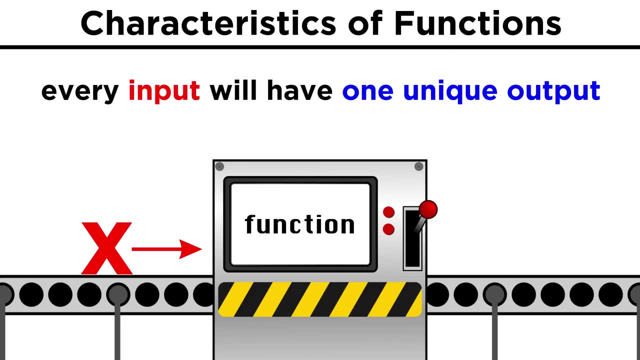 And so forth. We could make a table like this and we could even graph the resulting relationship. So everything we used to do with equations where y depends on x, we can do the same thing with functions. The only difference is that with functions, for any x value we plug in. there must only 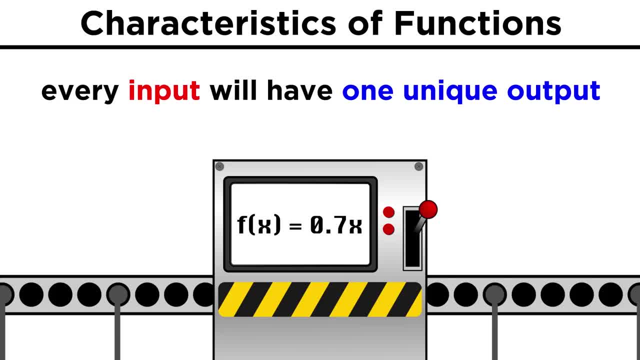 be one y value. For example, if a function tells us the sale price of an item, if we plug in the regular price we should get only one y value. So if we plug in the regular price, we should get only one y value. 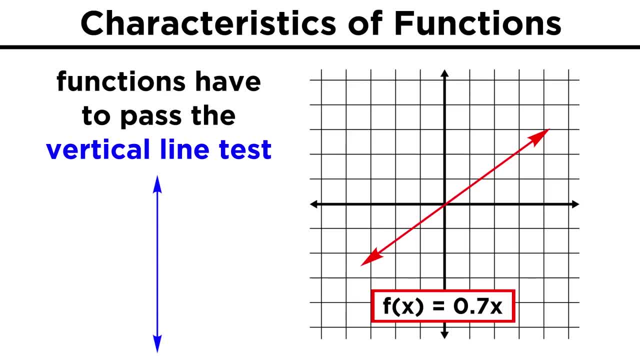 A function must pass only one sale price. For that reason, for a graph to be representative of a function, it must pass the vertical line test, Since a function can only have one output, or y value, for each unique input, or x value. 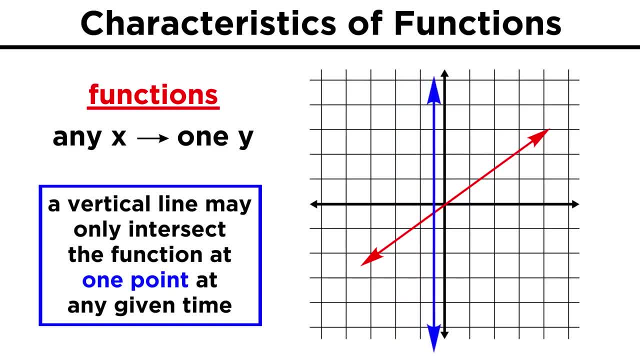 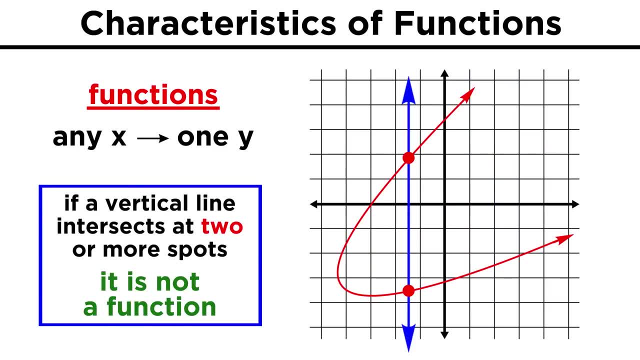 then if we move a vertical line across a function, it will only intersect that function at one point, wherever the vertical line may be. If the vertical line intersects at two points, we pass the vertical line test or more spots. it is not a function. 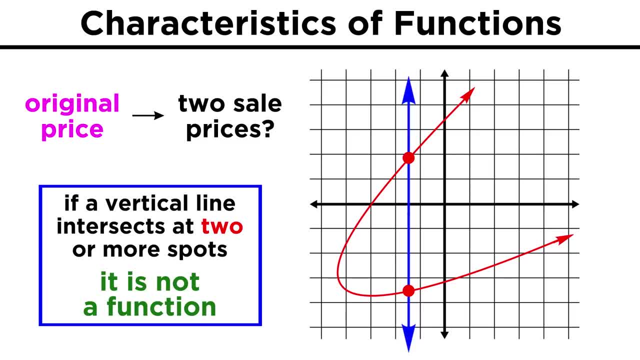 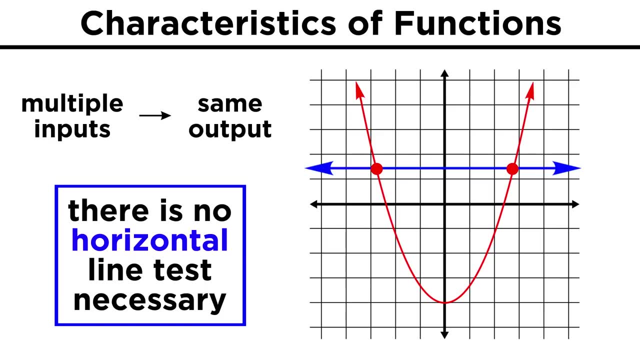 That would be as though we plugged in the regular price of an item and got back two different numbers for the sale price. We can, however, have the same output for multiple inputs, which is why different X values are permitted to produce the same value for the function. so there is no horizontal 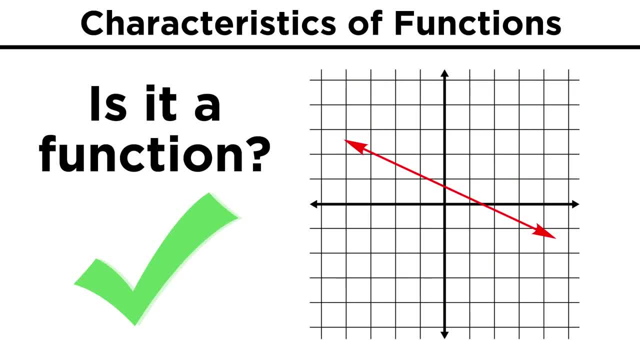 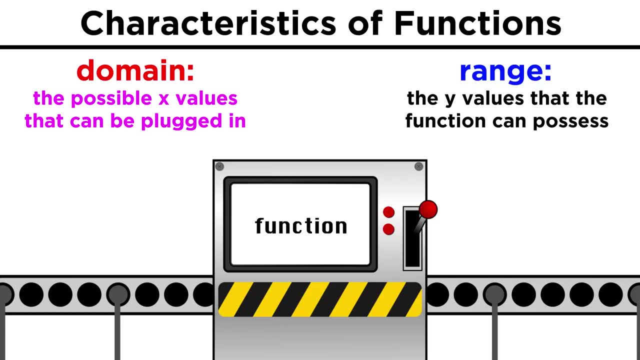 line test necessary. This line is a function. This circle is not. This curve is a function. This curve is not. We can also describe the domain and range of a function. The domain is essentially all of the values that can be plugged into the function. 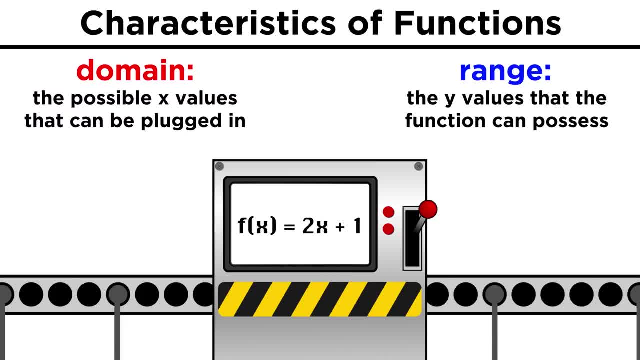 So if we have something simple like F of X equals two X plus one, the domain would be all real numbers or negative infinity to positive infinity. All the function does to the input is double it and add one, so any number will work. 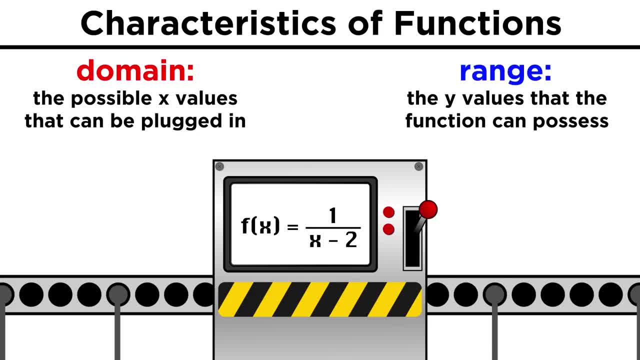 But there are examples where there are limitations to the domain. Let's say F of X equals one over X minus two. We can't divide something by zero, so X can't be two. If X was two we would get zero on the bottom and the function would be undefined. so two. 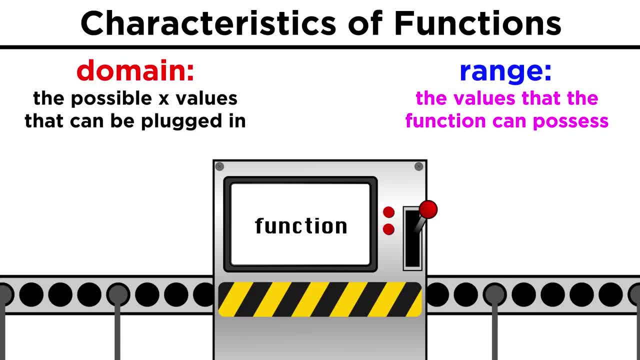 is not part of the domain. The range, on the other hand, is all the potential output values, or essentially the values that the function can possess. Again, something simple like F of X equals two, X plus one will yield a range that includes: 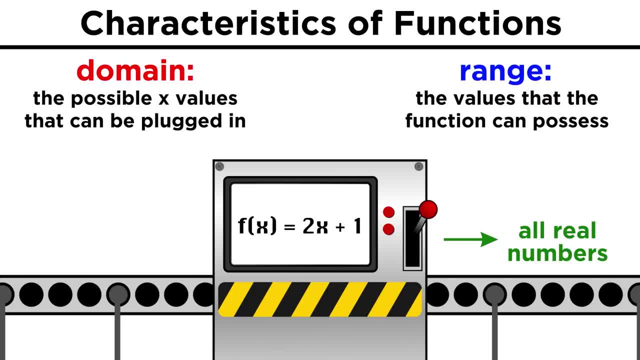 all real numbers, extending to infinity in each direction. But if we have something like F of X equals the absolute value of X, then the range is now limited to values greater than or equal to zero. The range, on the other hand, is all the potential output values, or essentially the values. 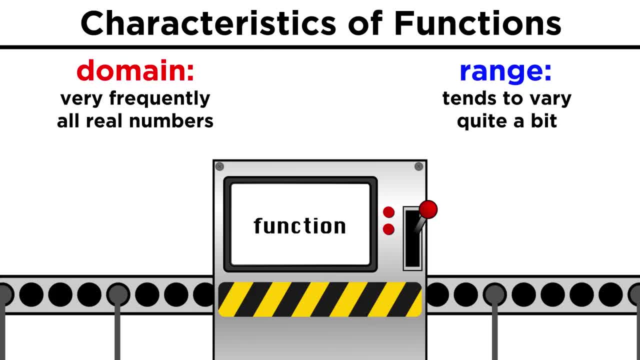 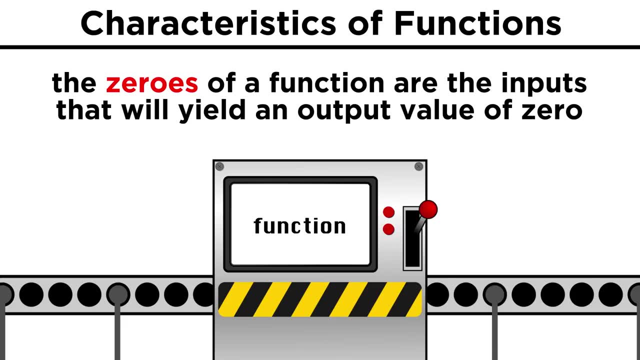 that the function can possess. So while the domain is very frequently all real numbers, the range has a tendency to vary quite a bit depending on the type of function we are looking at. We will also sometimes want to identify the zeros of a function. 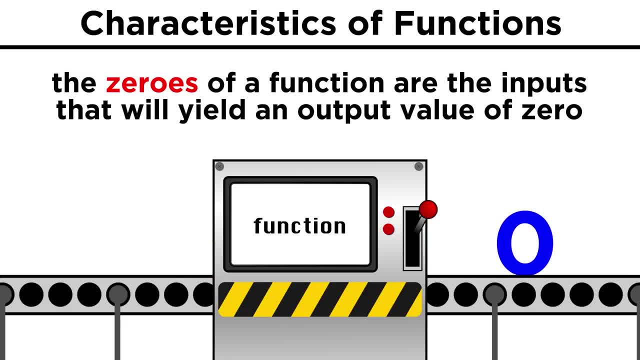 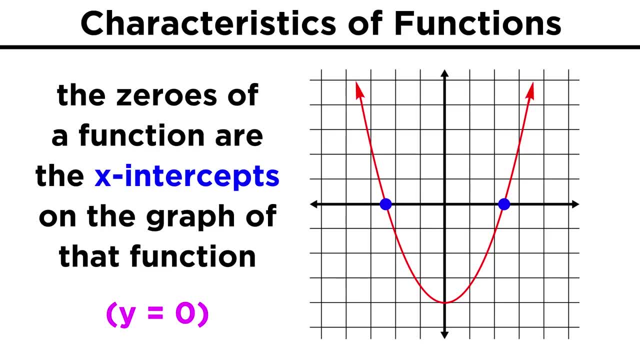 These are the input values that make the function equal to zero, which we can identify graphically as the X-intercepts. Wherever the function crosses the X-axis, we can identify the X-intercepts. That value of X is producing a Y value of zero, so that is a zero of the function. 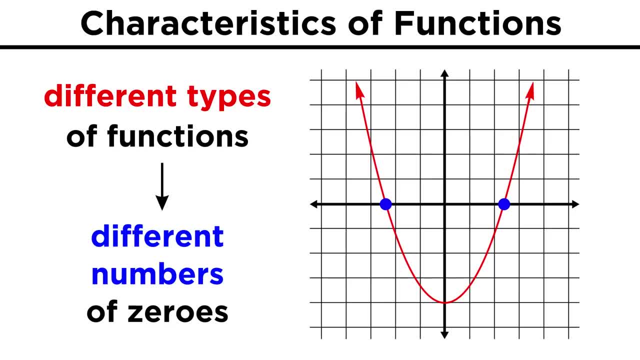 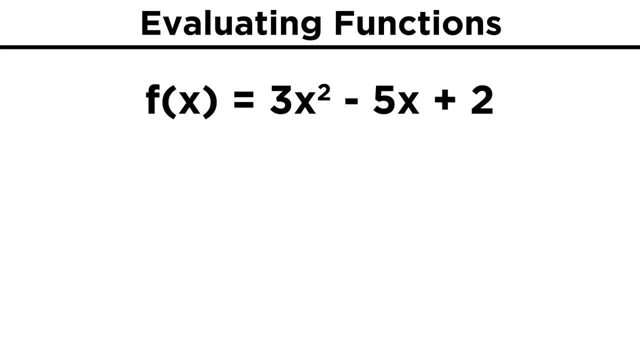 Again, different types of functions will have different numbers of zeros. Before we look at different types of functions, we need to make sure we know how to evaluate a function. For the function, three X squared minus five, X plus two, what is F of two?